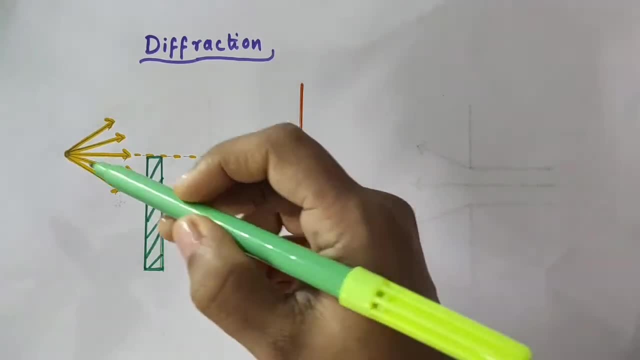 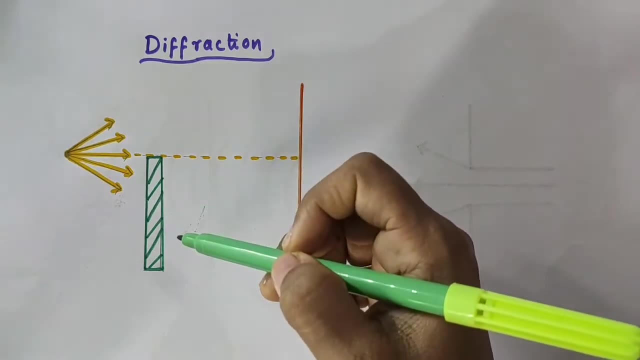 For example, consider an obstacle here and a point source of light here. Obstacle is just an object or thing that blocks the rays of light here. Okay, it is an opaque object. We have kept a screen here. Okay, this is the screen. 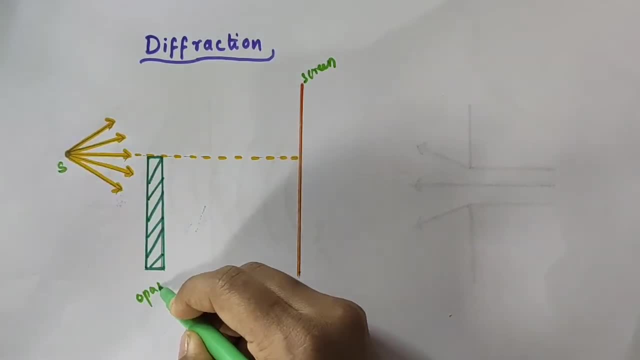 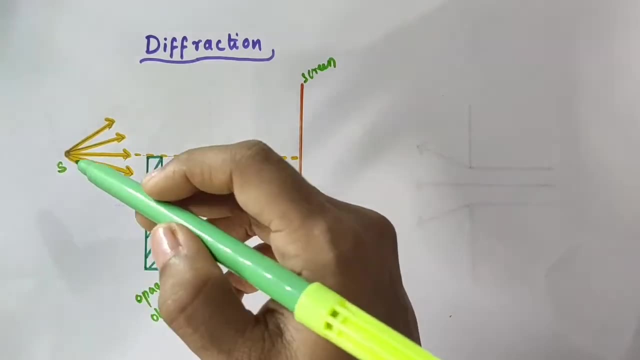 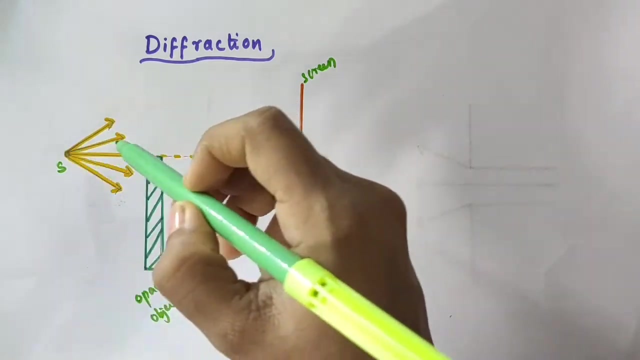 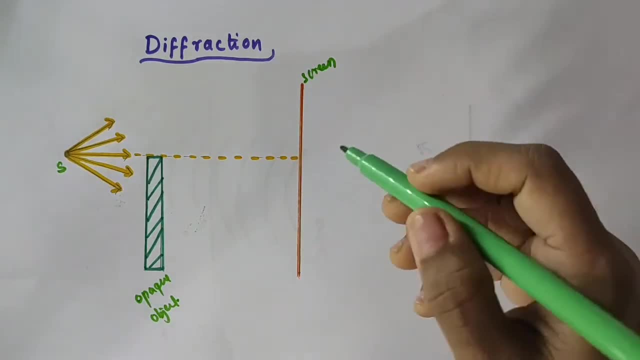 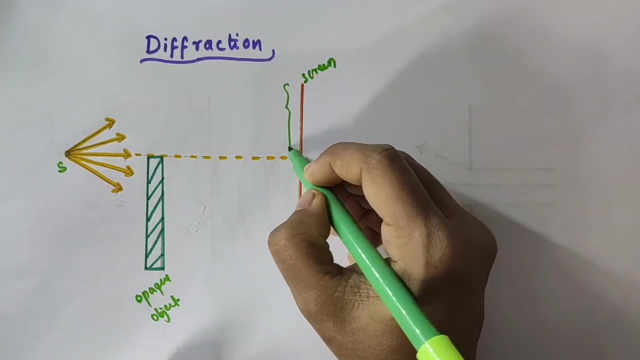 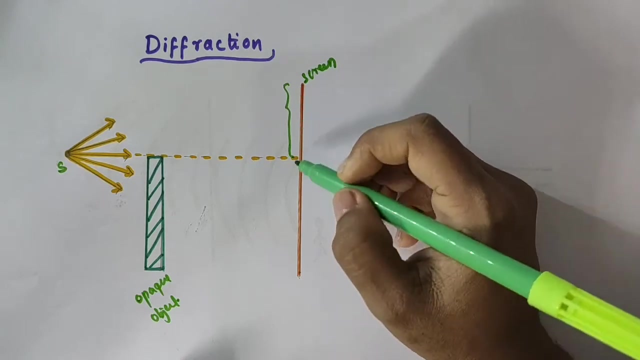 What do we expect here? actually, We expect the light reaches here. Okay, we expect the light reaches here, in this region. We expect the light reaches here, that is, in this region. That is, light reaches to this part of the screen and we will get a bright region of light here or an illuminative region of light here. 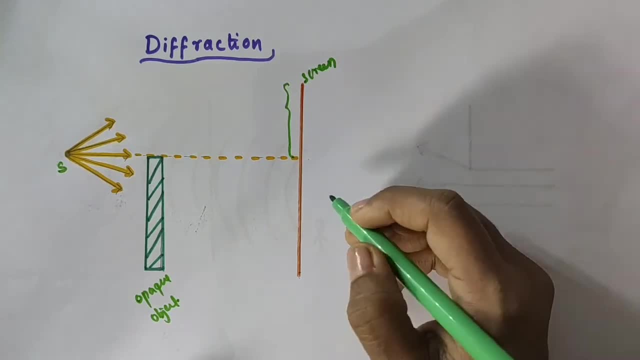 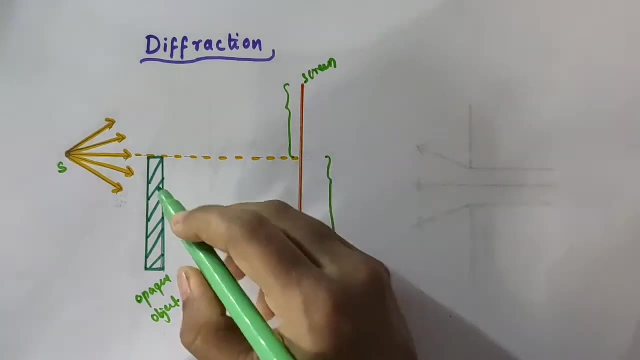 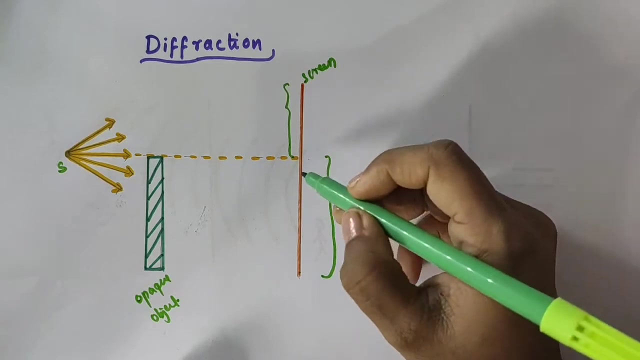 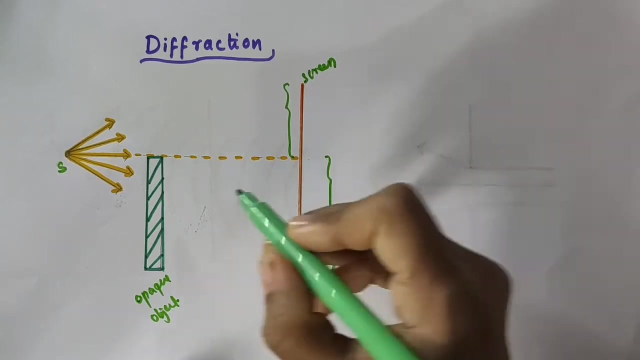 And we expect a shadow of this opaque object from here onwards. Okay, we expect a shadow of the opaque object from here onwards, Okay. that is, we expect a dark region from here onwards on the screen, Because we used to say that light seems to travel in a straight path. 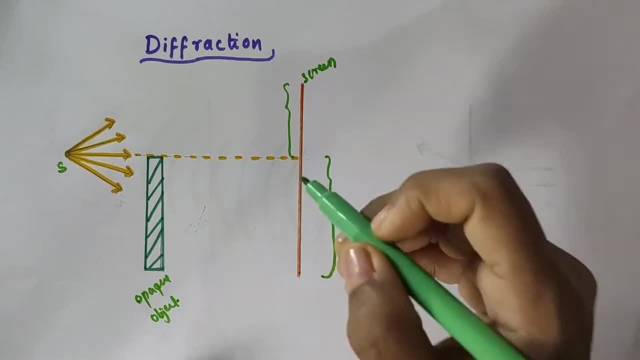 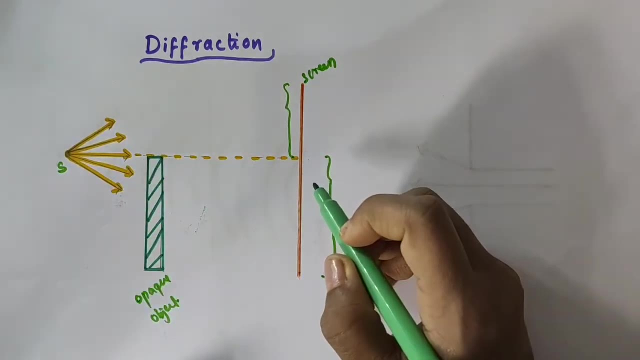 But this straight line approximation or straight path approximation is applicable only when we consider the particle nature of light or light rays. Okay, this straight line approximation is invalid When we consider the light as a wave, But what really happens is we will get a shadow. 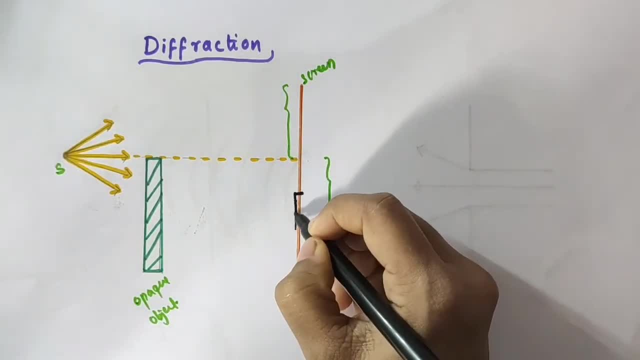 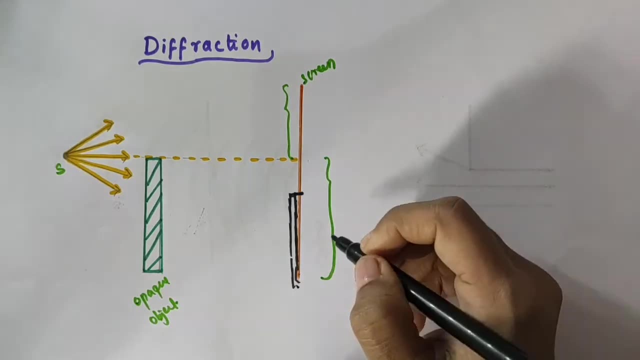 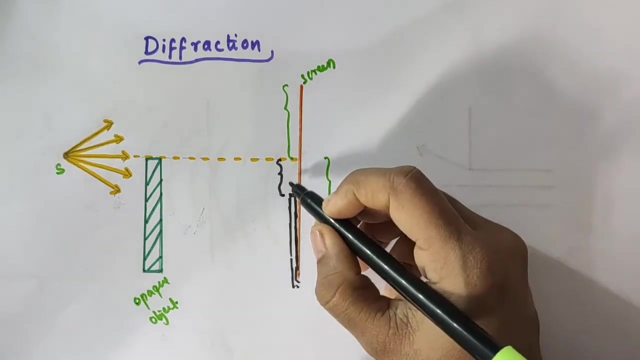 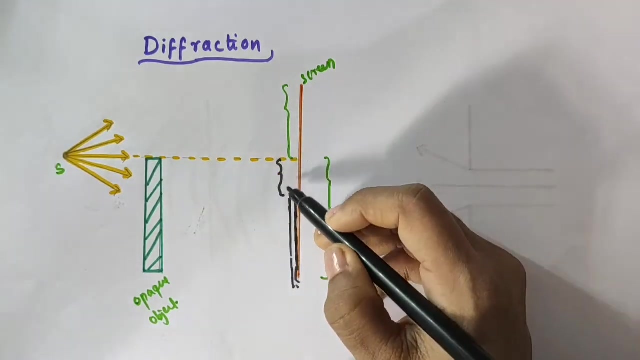 region from here onwards. Okay, we will get a shadow region from here onwards. Okay, that means light reaches to this region too. Okay, that is, light enters to this region. That is, light enters to the region of geometrical shadow, of this opaque object. 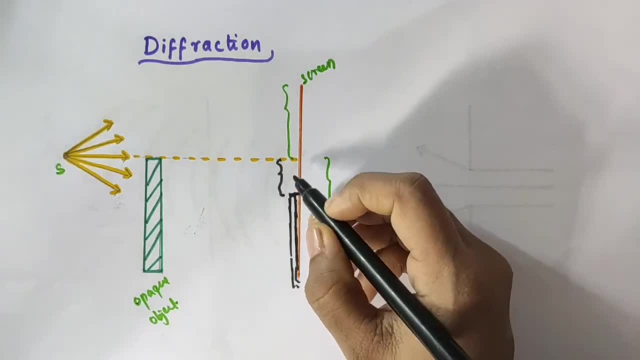 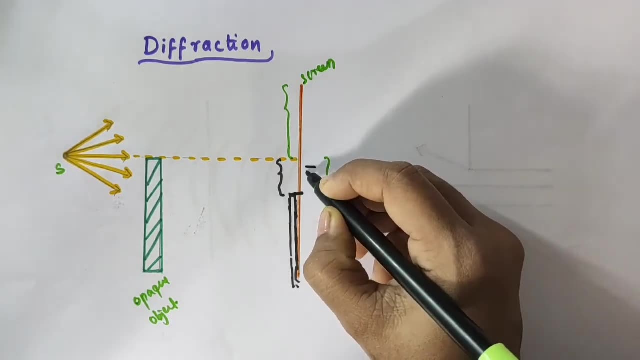 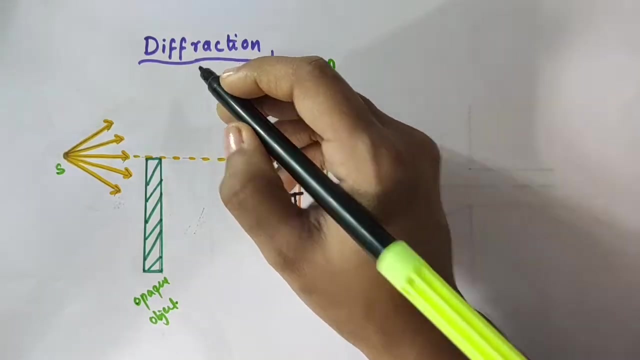 Okay now if we look clearly at the shadow caused by an opaque object close to the region of geometrical shadow, there we can see the alternate dark and bright regions. just like interference, This happens due to the phenomenon of diffraction. Diffraction is exhibited by: 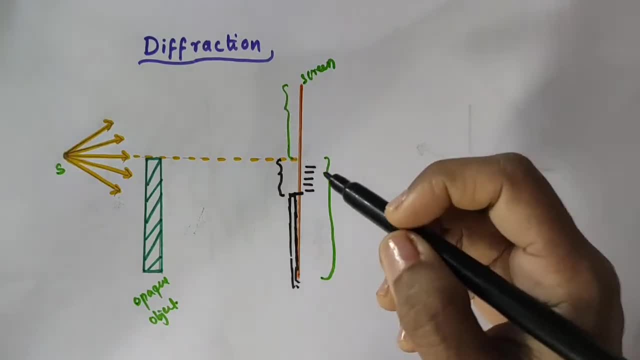 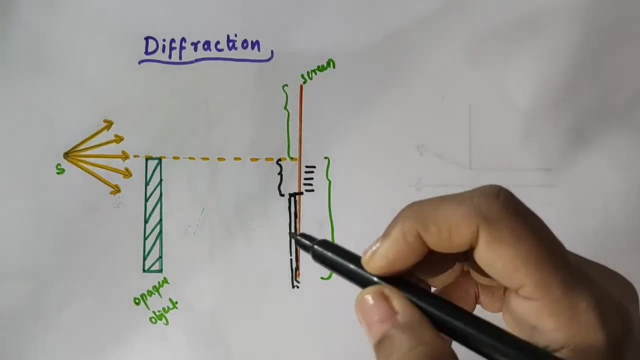 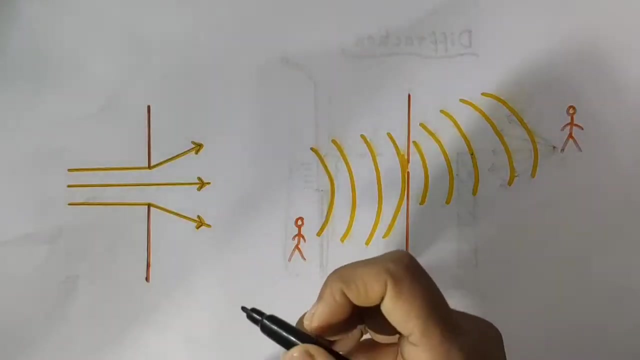 all types of waves, like sound waves, light waves, water waves, matter waves, atmosphere places. Since wavelength of light is much smaller than the dimensions of most of the obstacles, we do not encounter diffraction effects of light in everyday observations. The finite resolution of our eye or of optical instruments such as telescopes or microscopes is limited due to the phenomenon of diffraction. 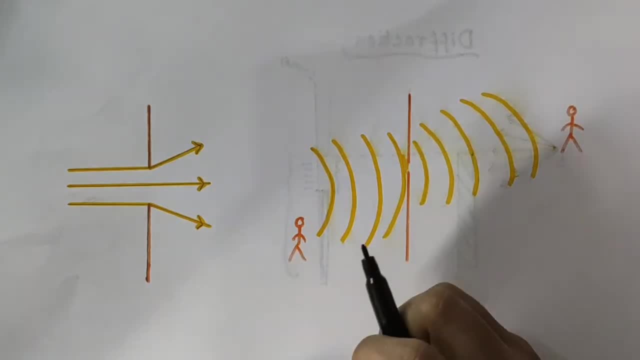 Due to diffraction of light, the image of a specimen never perfectly represents the real details present in the specimen, because there is a lower limit below which the microscope or an optical system cannot resolve structural details. The colors that we see when a CD is viewed- compact disc, CD is viewed due to that is actually due to that. colors is actually due to diffraction effects. 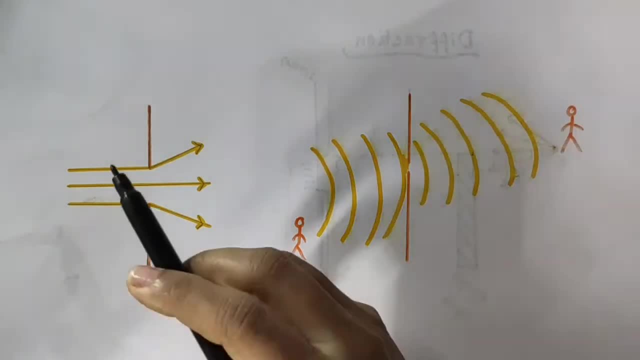 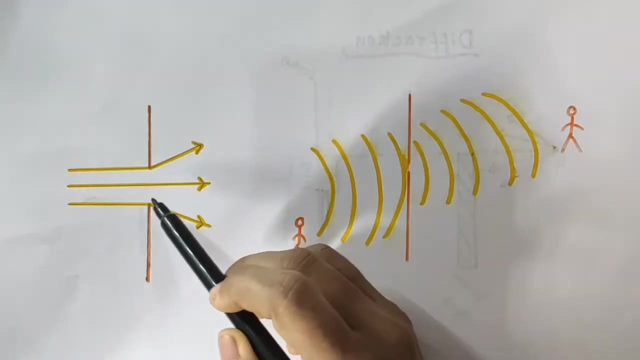 The color we see is the diffraction pattern, actually The effects of diffraction. Diffraction can only be properly understood using wave ideas. Diffraction involves the change in direction of waves as they pass through the opening or around the barrier in their path. 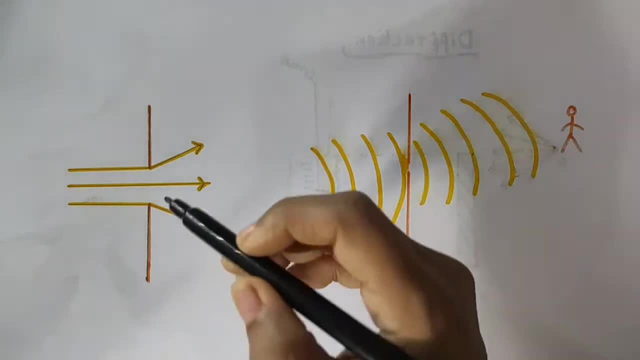 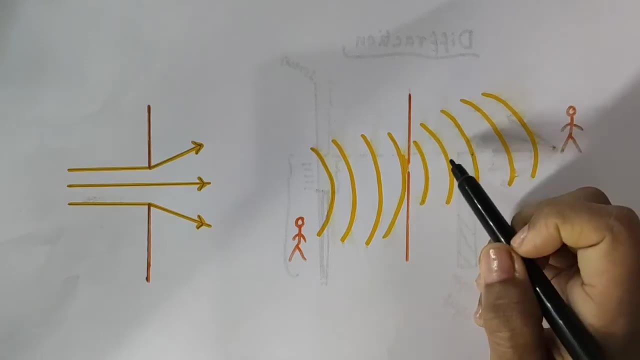 When the wavelength of the wave is smaller than the obstacle or opening, no noticeable diffraction occurs. Diffraction of sound waves is commonly observed: Sound diffracts around the corners of door openings, Sound diffracts around the door openings And allowing us to hear others who are speaking to us from adjacent rooms. 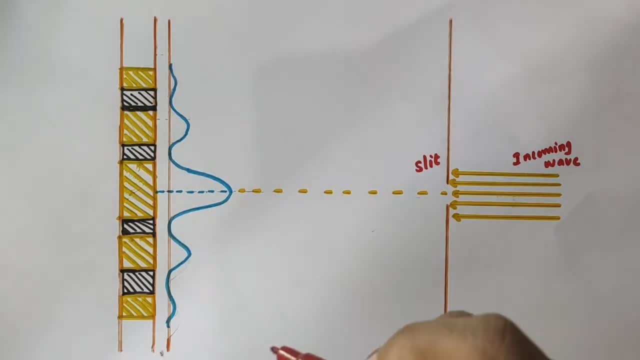 While we have discussed about Young's Double Slit Experiment, we considered two narrow slit snow and they were illuminated by a monochromatic source of light. I will provide a link for that Young's Double Slit Experiment in the description box. if you want, you can watch that. 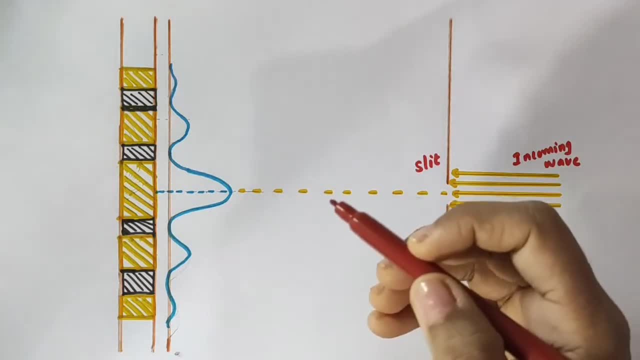 Now when the double slit in Young's Double Slit Experiment is replaced by light? Now when the double slit in Young's Double Slit Experiment is replaced by light, by a single narrow slit and illuminated by a monochromatic source, let us see what happens. 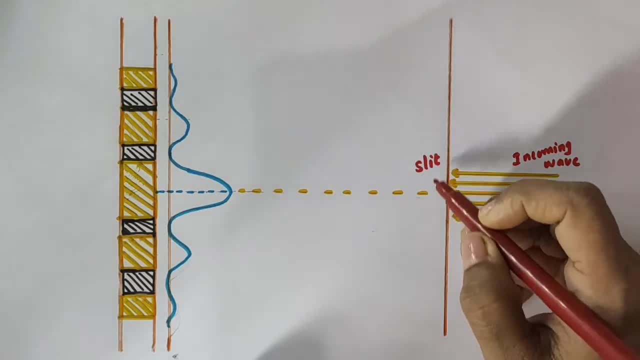 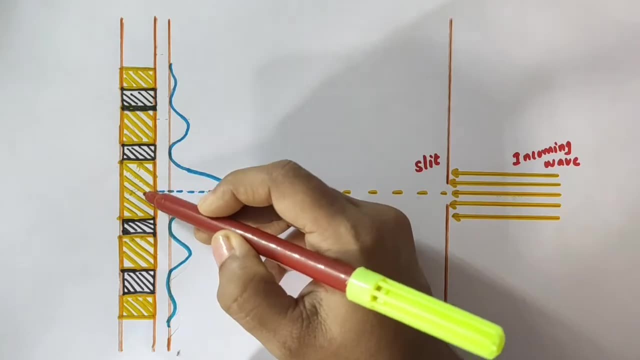 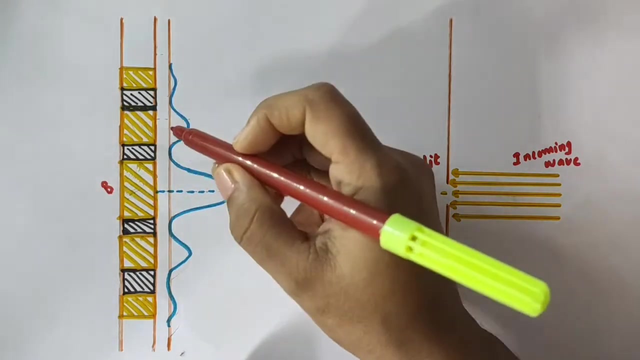 see. when a single narrow slit is illuminated by a monochromatic source of light, a broad pattern with a central bright region is seen on the screen. okay, this is the central bright region. okay then, on both the sides there are alternate dark and bright regions and intensity you can see. 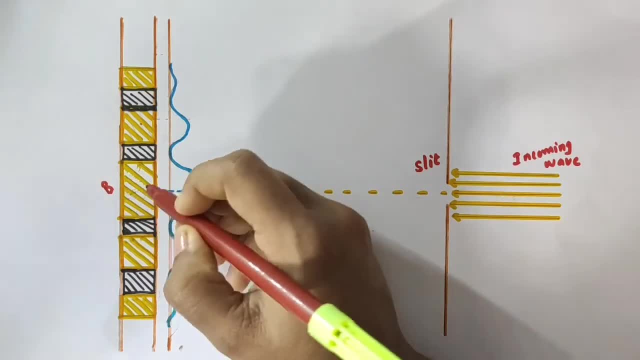 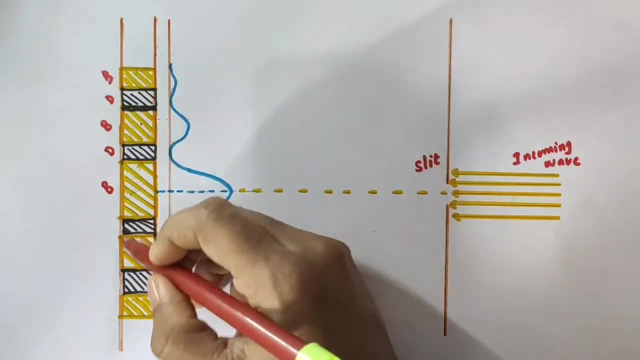 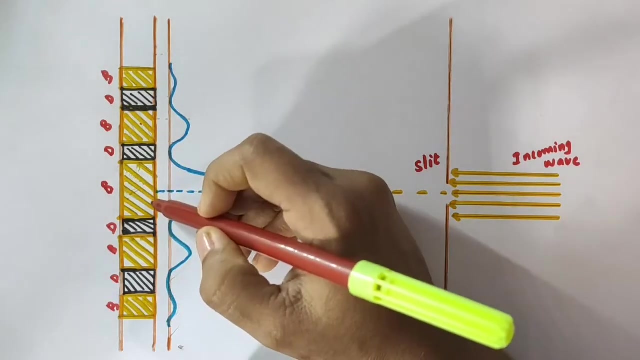 that intensity becomes weaker. okay, so we have the central bright region, then alternate dark bright, dark bright regions to this side and here also dark bright, dark bright regions on this side. okay, and you can see that the intensity becomes weaker when, when we move away from the center. 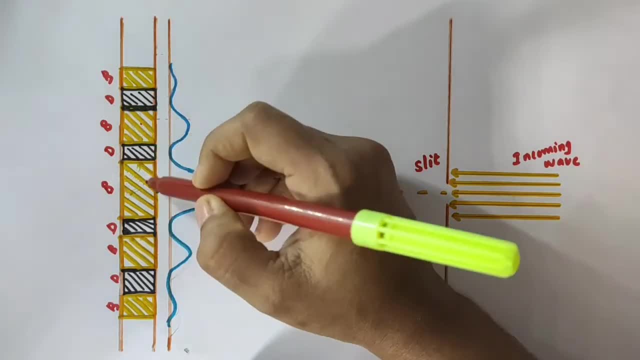 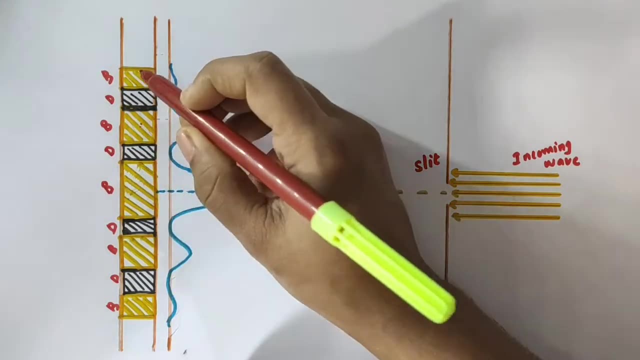 see central bright region on this side and here also dark, bright, dark, bright regions on this side. bright region: okay, quite intense. but you see, when we are moving away from the center, intensity you can just compare the intensity with the thickness of this region. okay, here intensity decreases, here also intensity becomes weaker. 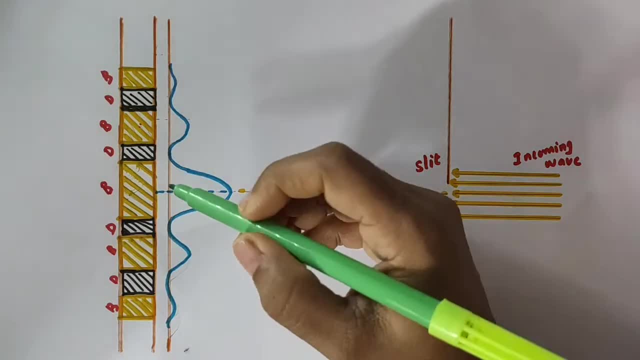 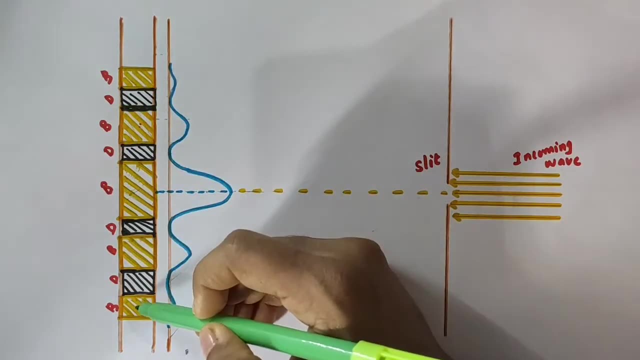 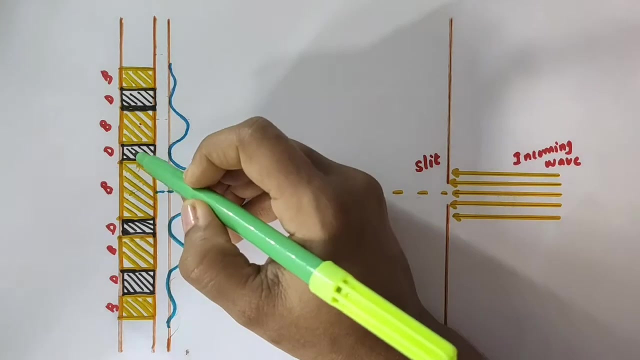 that is, here we will get a very bright region, and brightness decreases when we consider points away from the center. so, corresponding to these, we will get bright spot or bright fringe. and corresponding to this, we will get bright spot or bright fringe. and corresponding to this, we will get 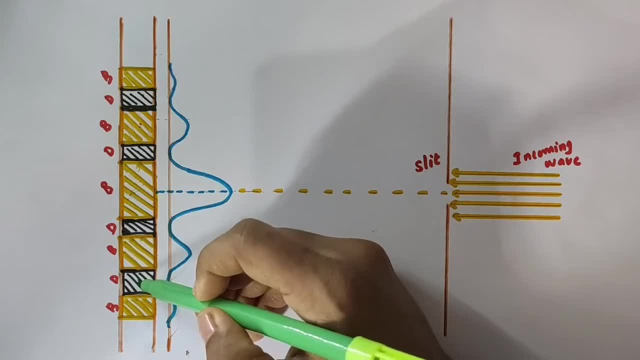 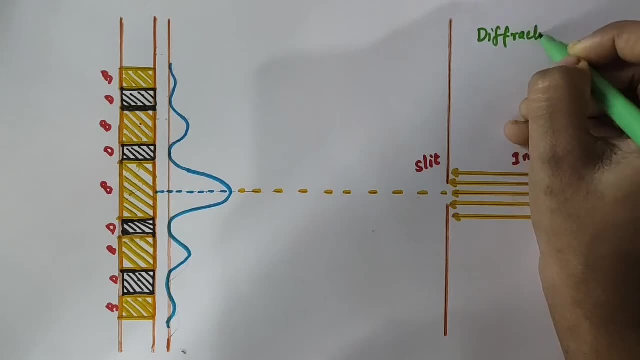 bright spot or bright fringe and corresponding to this, we will get bright spot or bright fringe. and contrasting to this, we will get dark spot or dark fringes. okay, the brighter dark fringes are, Okay, the right end dark fringes are called as diffraction fringes- okay. 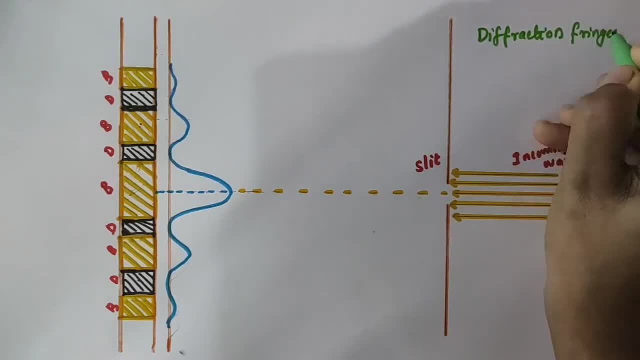 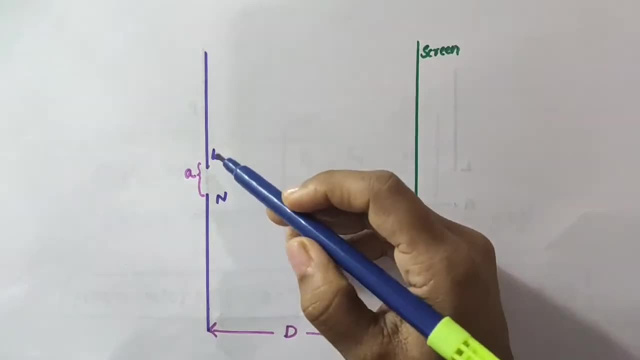 Gleicher the darker. i mean brighten, dark fringes are called as diffraction fringes. Now know, consider a single slit L here of width a screen is kept here. Now let's chapter a. go over Here we have double-slit Ln width a. we have our solid width of ln here. and what is this area which is? 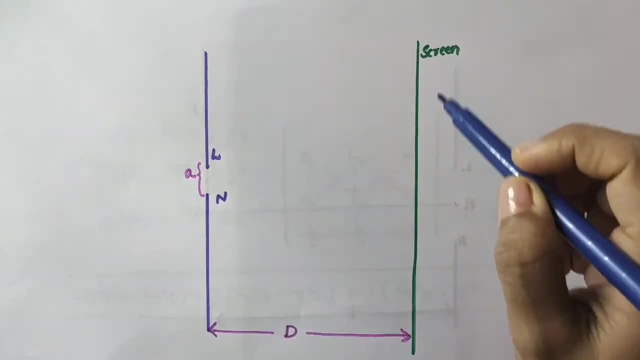 Capilator D be the distance between the slit and the screen. The slit is practically very small, such that A is less than less than capilator D. That is capilator D. this distance is very much greater than the width of the slit. 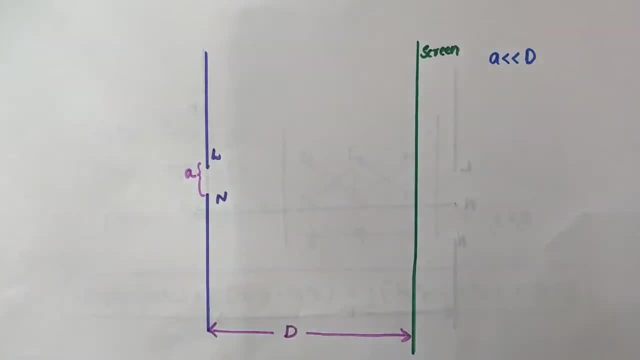 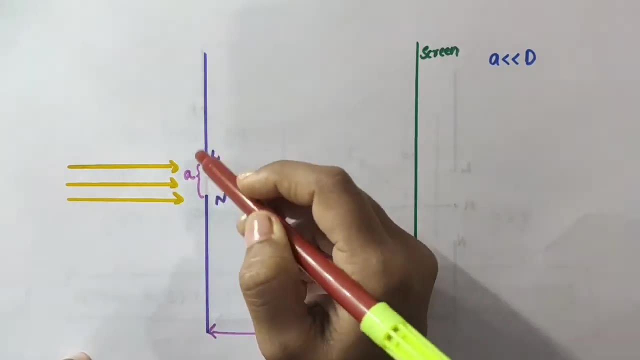 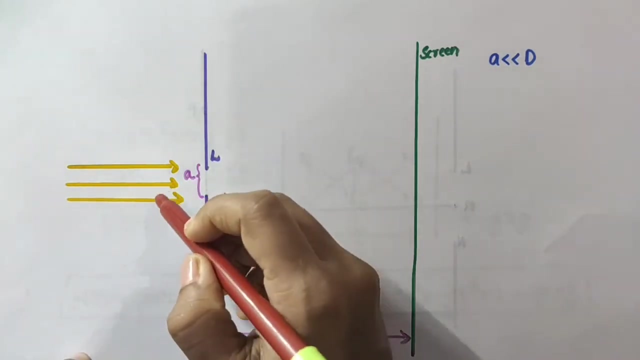 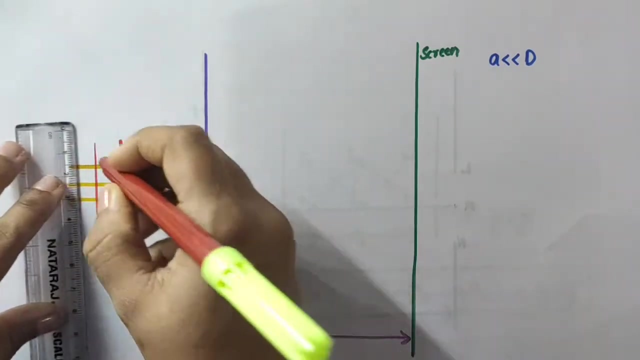 Okay, that is, the slit is practically very small. Now consider a parallel beam of light falling normally on the slit: LN of width. small letter: A Parallel beam of light means what Their corresponding wave fronts are plane wave fronts. no, Okay, their corresponding wave fronts are plane wave fronts. 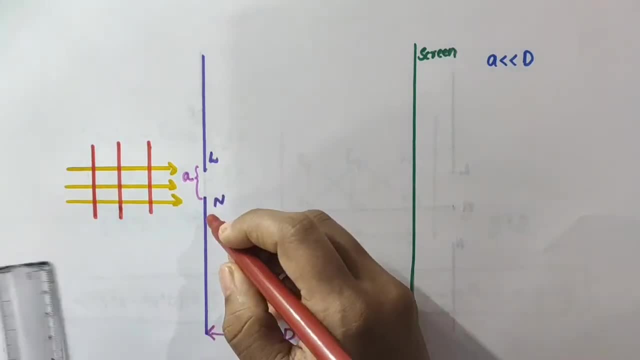 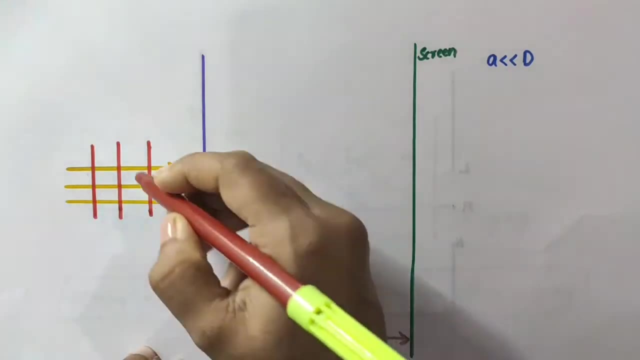 Okay, their corresponding wave fronts are plane wave fronts. That is, incoming wave front is actually parallel to the plane of the slit. This is the wave front. This is actually the parallel beam of light. So corresponding to that, their wave fronts will be, I mean, like this: 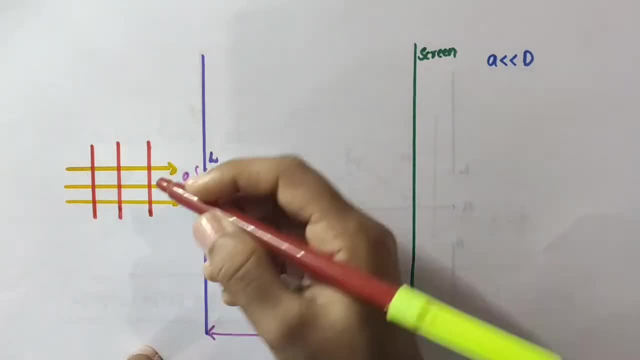 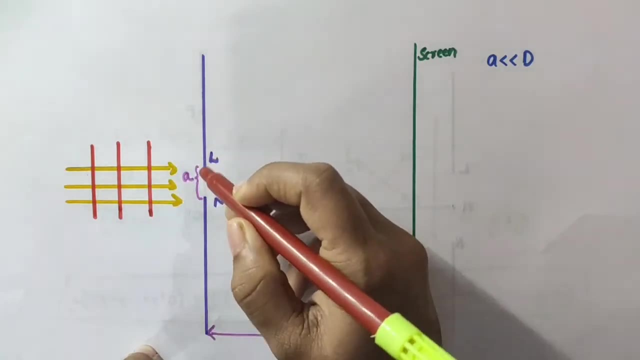 Which we have discussed in our previous videos. I hope you remember this. We will get plane wave fronts here, And the incoming wave front is actually parallel to the what, the plane of the slit. Okay, and hence each on that plane wave front, each point on that plane wave front, will be in face. 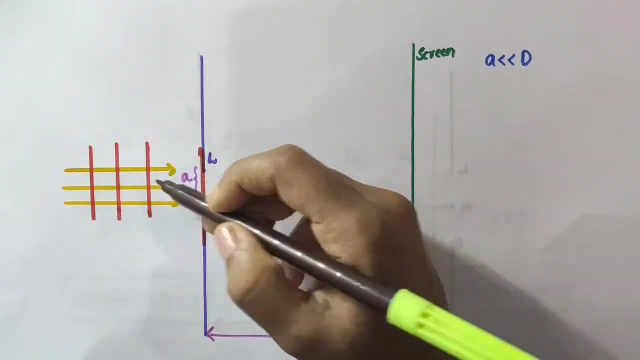 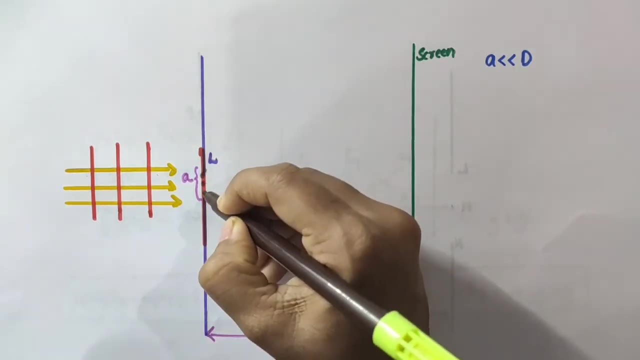 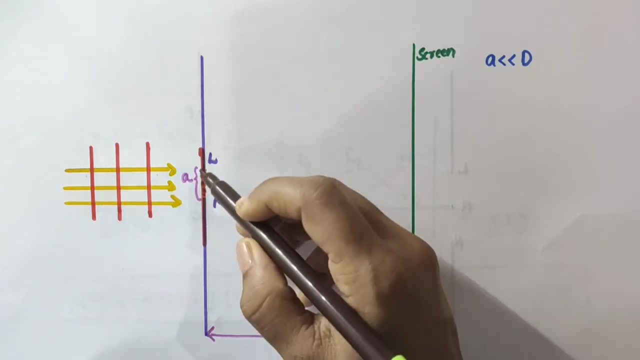 Okay, when this wave front reaches at the slit, We can consider so many points On the wave front. Okay, we can consider so many points on the wave front at the slit. Okay, and each point on the wave front You can consider point here: 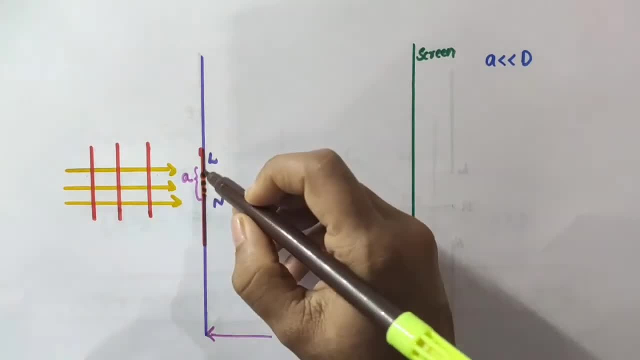 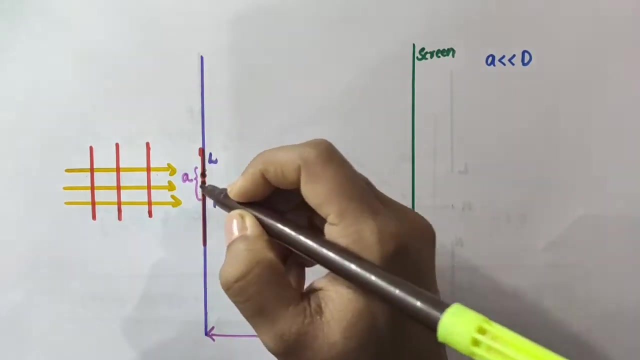 You can consider point here. You can consider point here. We can consider a point here. We can consider so many points on the wave front and each point on the wave front at the slit will behave like a secondary source. Okay, each point on the wave front at the slit will behave like secondary sources. 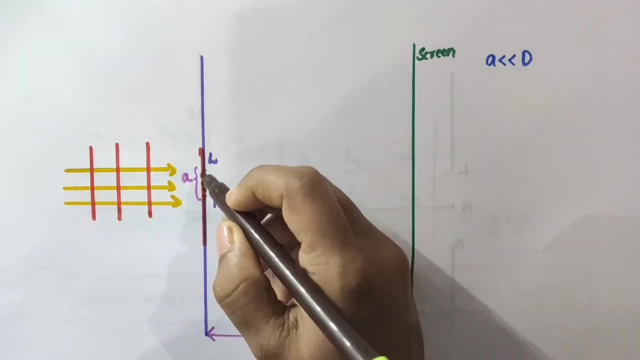 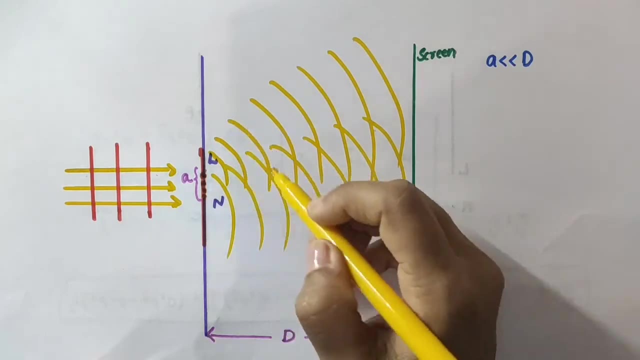 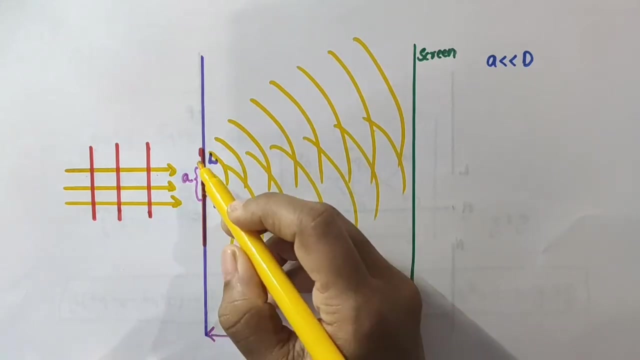 That is, We can treat the different parts of the wave front at the slit as secondary sources. So secondary wavelets are emanating from each point on the wave front. Okay, each point on the wave front at the slit, Secondary wavelets will emanate from this point, from this point. secondary wavelets from will emanate from this point, this point, etc. 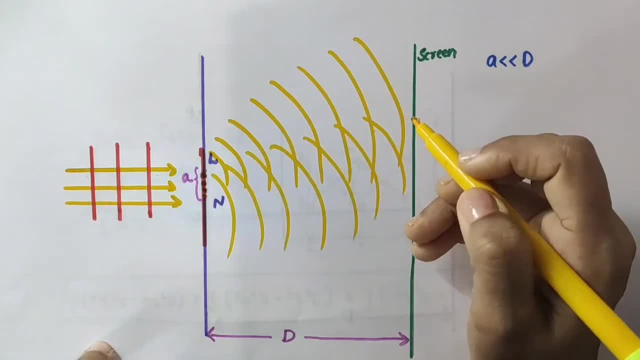 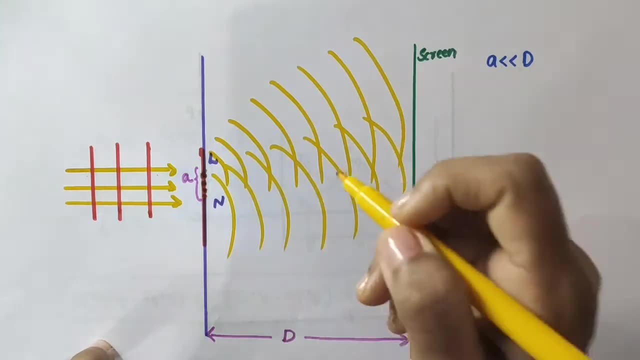 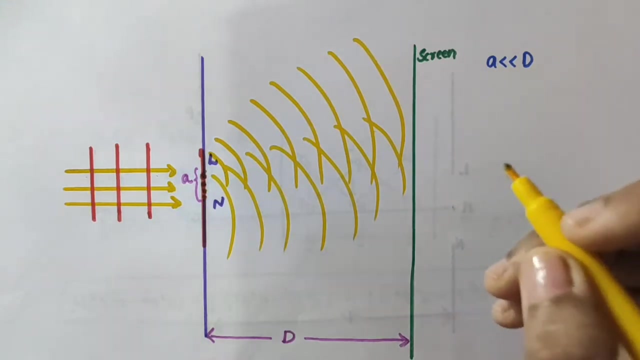 And at some points constructive interference takes place and we will get bright spot or bright fringe at that point and at some points destructive interference takes place. corresponding to that, we will get dark fringes. While we have discussed about Young's experiment and interference fringes, we considered two slits and each slit was acting like a source, and only two sources were there. 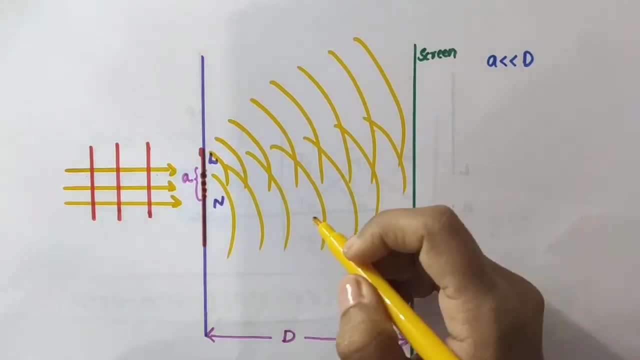 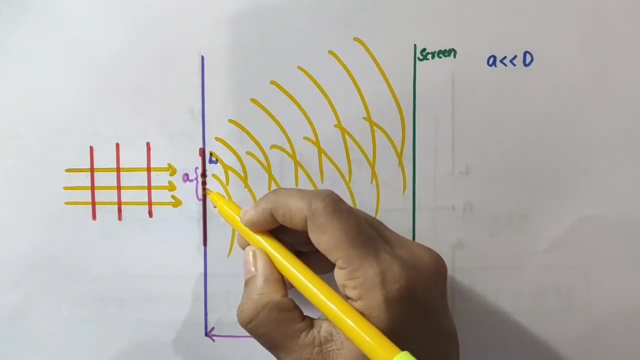 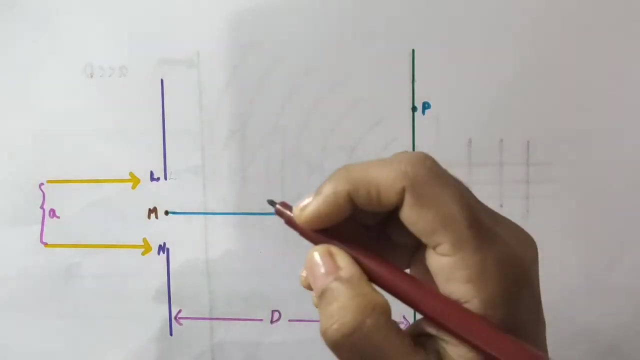 But, But, But. But. Here you see, we have only one slit, Okay, and we have so many number of sources, Okay, in the case of diffraction. Now let us consider the midpoint of the slit. The slit is Ln. 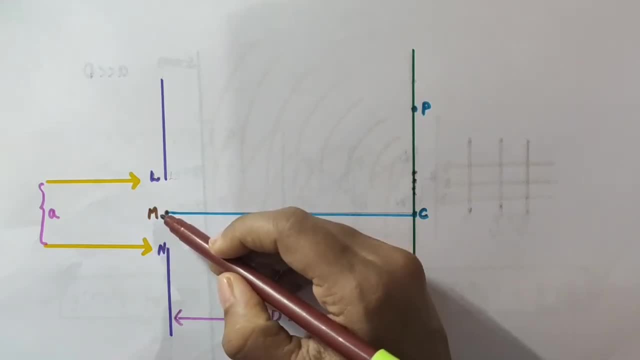 So let us consider the midpoint of the slit. I have just named it as capilator M- Okay. let us consider a straight line through M? Okay, and perpendicular to the slits. The slit is like this: This line through M is actually perpendicular to the slit. 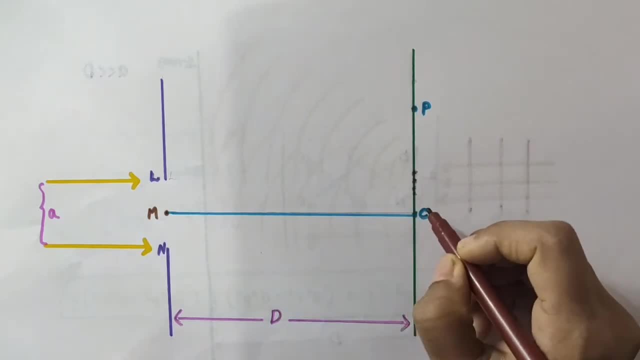 Okay, then this line meets the screen at this point. Let this point be capilator C, So Mc is actually the perpendicular bisector of the slit Ln. Okay, we want the intensity at any point- P on the screen. This is the screen. 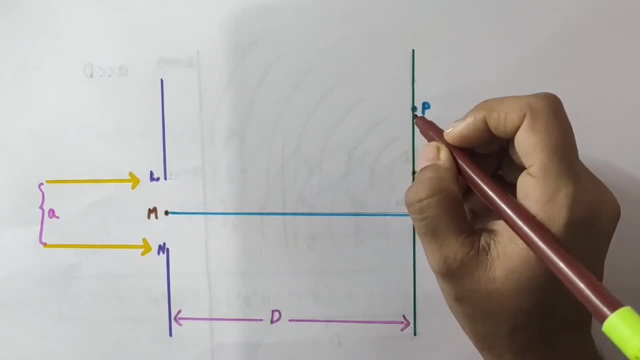 And this is, you can take any point. Okay, this is just like an arbitrary point taken on the screen. We want the intensity at any point P on the screen, Okay, so let that point P be somewhere here. You can consider the point here. 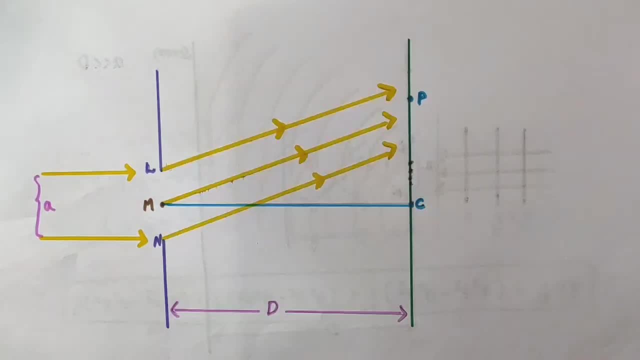 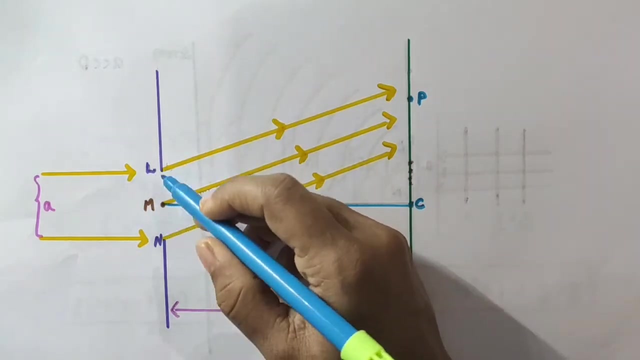 You can consider that point here. It's up to you. Alright, The straight lines joining P to the different points, L, M, N, etc. can be treated as parallel. You can consider so many other. You can consider so many other points in between these two. 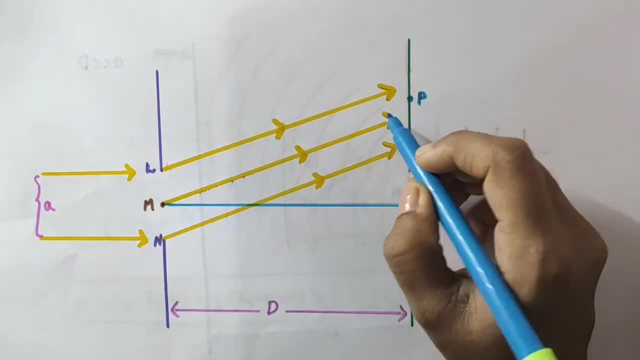 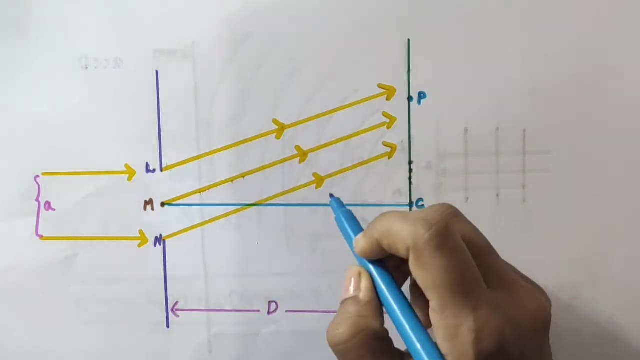 Okay, the straight lines joining to the different, I mean joining P to the different points, L, M, N, etc. can be considered, can be treated as parallel. See, the screen is kept very far away from the slit, So D is very large. 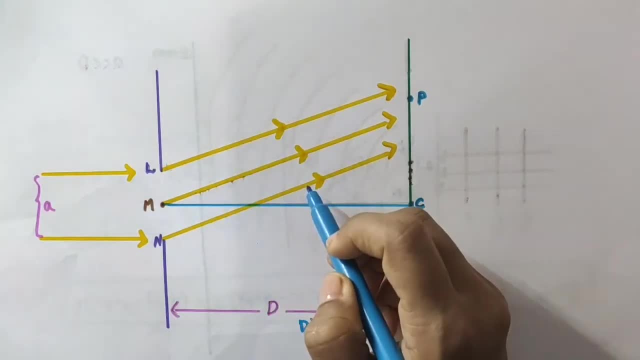 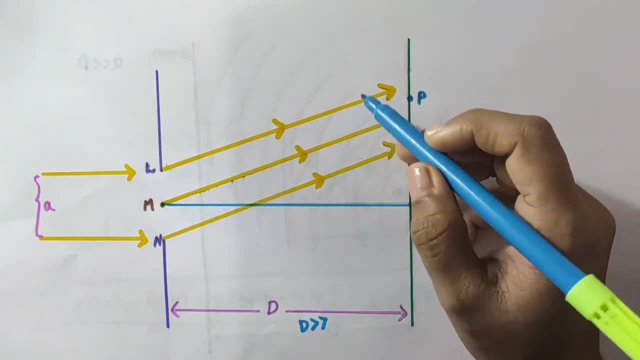 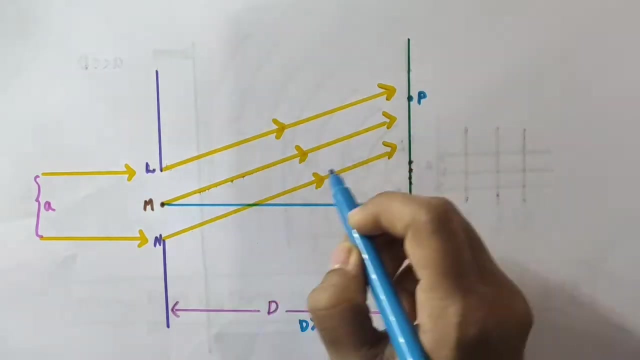 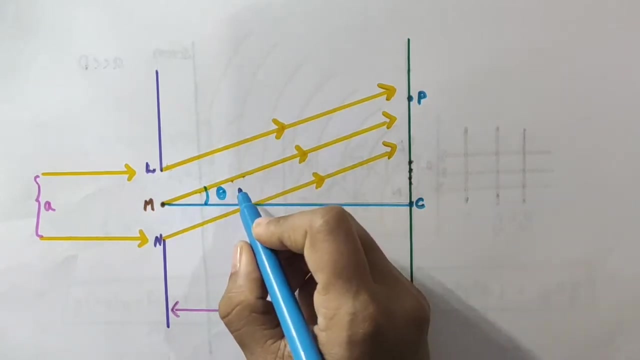 Okay, so we can consider these rays of light corresponding to the wave front as parallel, like this: Okay, we can make use of a convex lens here to converge these rays to the point P on the screen. Now let these lines make an angle theta with the normal. okay, let these, I mean let these lines, make an angle theta with the normal line MC. 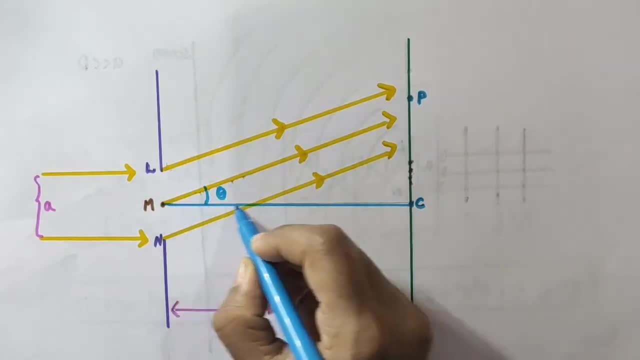 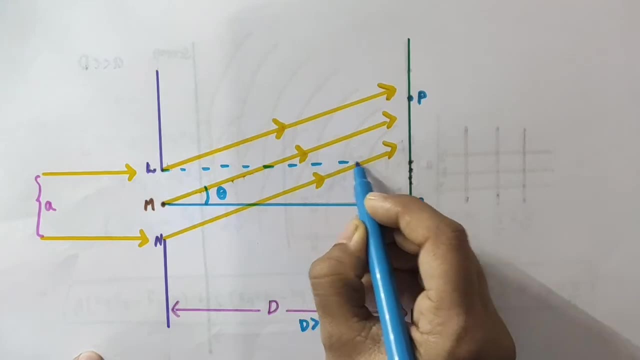 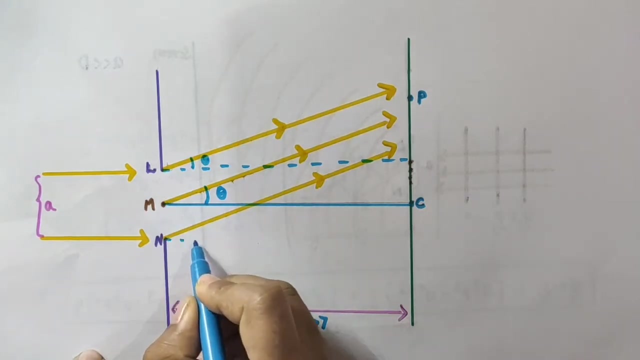 Okay, so this line actually makes an angle- theta- with this normal line MC. Similarly, if I, We can just consider a parallel line here which is parallel to this MC, So this angle also would be theta. Alright, Similarly, we can consider a line which is parallel to MC here: 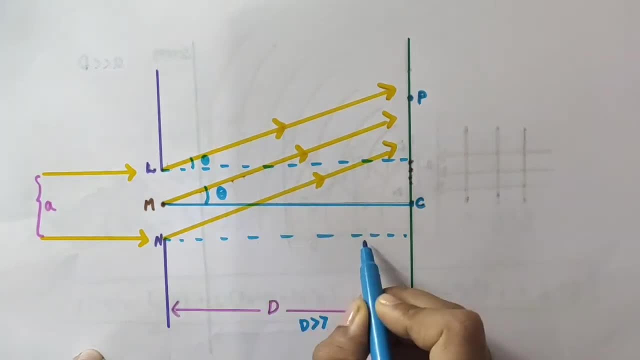 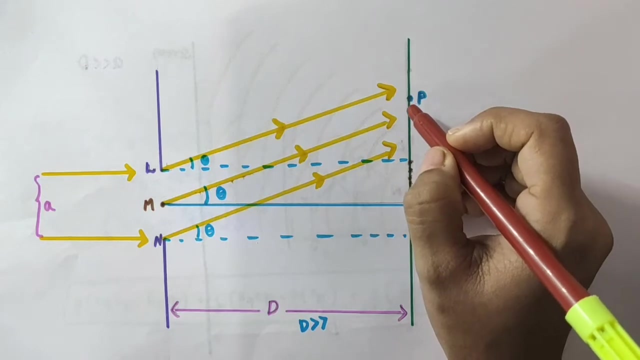 Okay, So this is parallel to this and this line is parallel to this. So this angle also would be theta. Okay, Now, what is the path difference between the waves at the edges to the point P? Path difference between the waves at the edges. 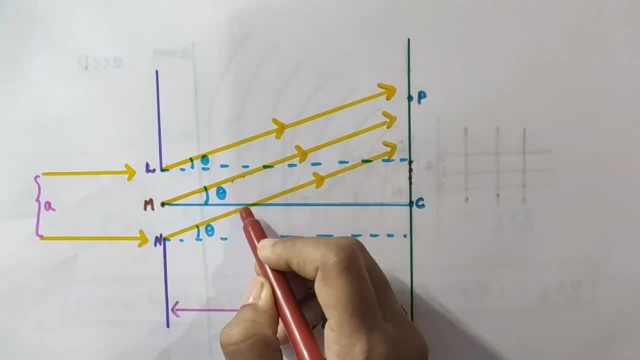 That is path difference between this wave and this wave. Okay, What is the path difference between the waves at the edges to the point P? See, this wave has travelled this much distance and this wave has travelled quite more distance than this. Okay, 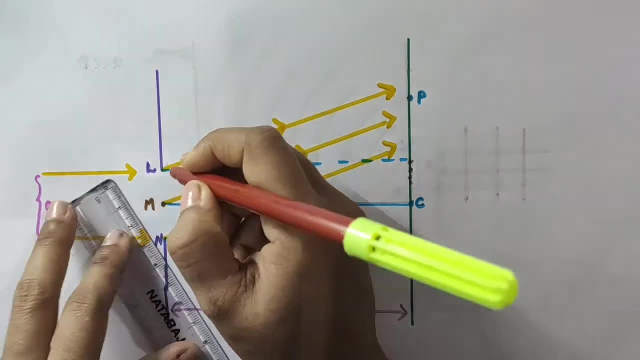 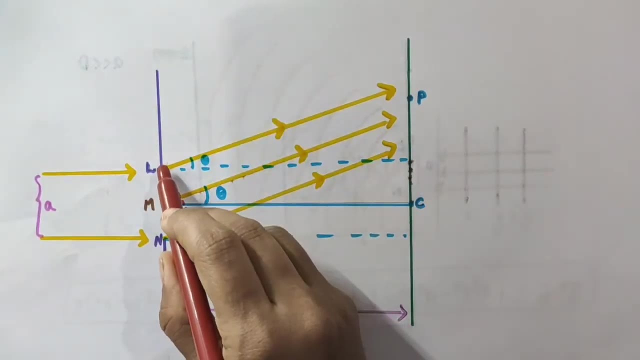 See, I am just So, I am just drawing a line here. Okay, I am just drawing a perpendicular line here So you can see that the path travelled by this is this and, path travelled from here, the wave is actually this much. 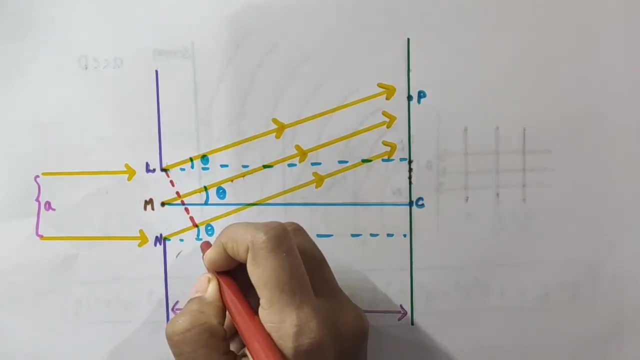 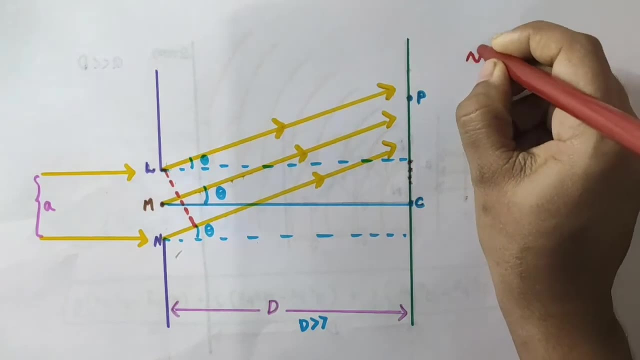 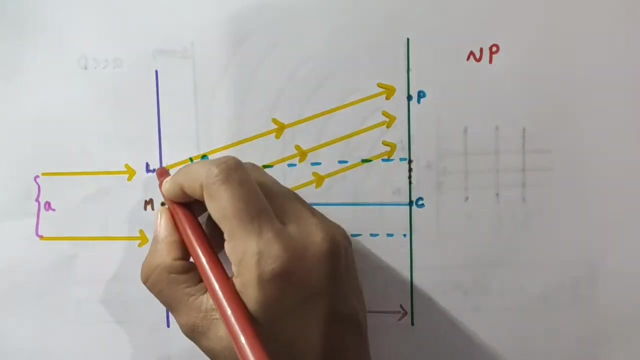 So there is this much path difference between these two. Okay, That is actually. we want to calculate NP minus LP. Okay, NP is the path travelled by this wave from this, And LP is actually the path length travelled by this wave from this edge. 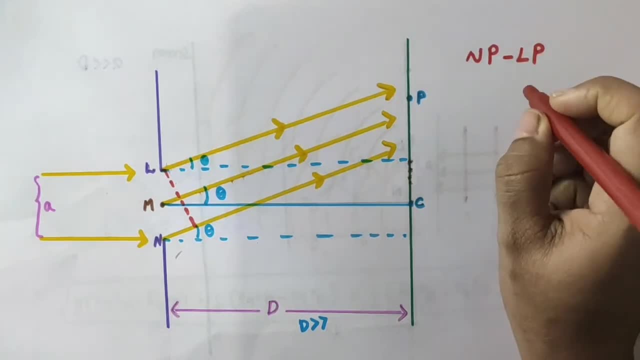 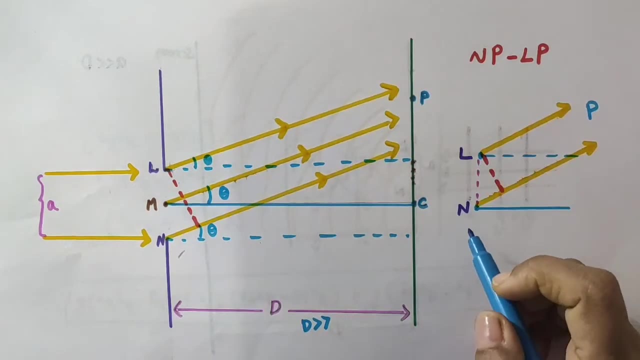 So NP minus LP is actually the path difference between the two edges of the slit. See here, I have just redrawn this figure here. Okay, See, the waves from the edge L of the slit and the wave from the edge N of the slit are travelling different path lengths to reach the point. 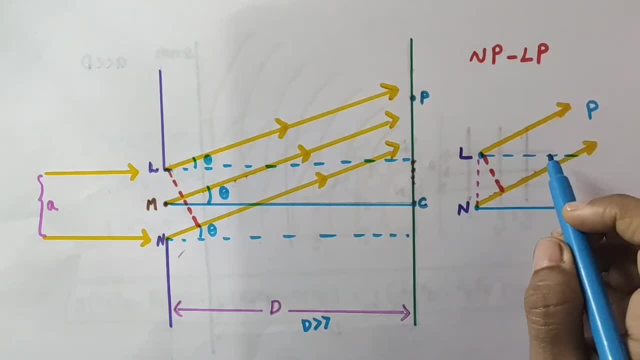 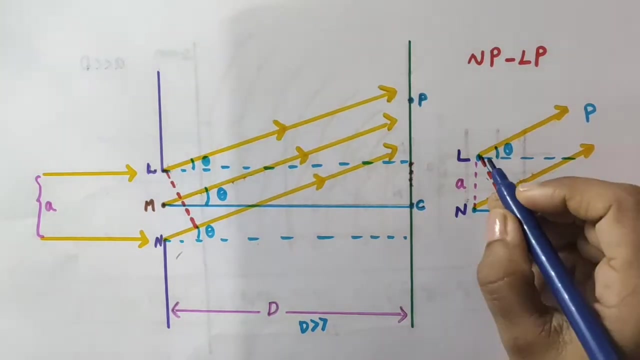 So to find out the difference in path, I have just drawn a perpendicular line from the point L to this line NP And let this point be Q. So the path difference NP minus LP between the two edges of the slit can be written as what: 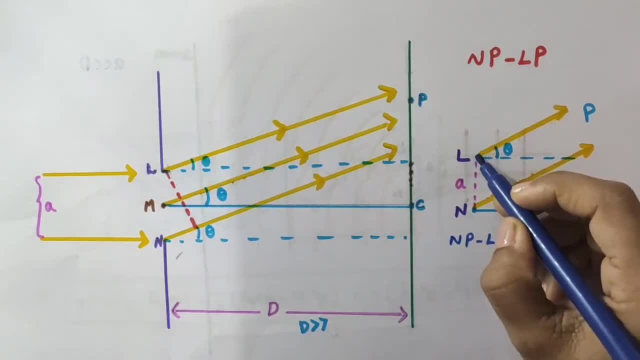 NQ. Okay, That is. the Wave from this edge has travelled this much distance. Wave from this edge has travelled this much distance. So there is this much path difference between the path length travelled by these two waves. So that path difference is actually equal to what? 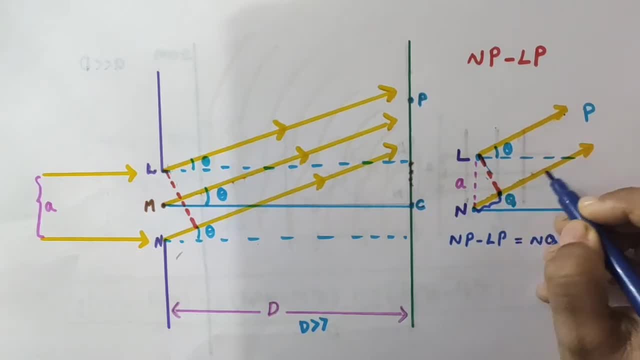 NQ. That is, from this point to P and from Q to P, the path lengths are the same. Okay, So there is a difference of this much between them. That is NQ. So we can write: the path difference: NP minus LP is equal to NQ. 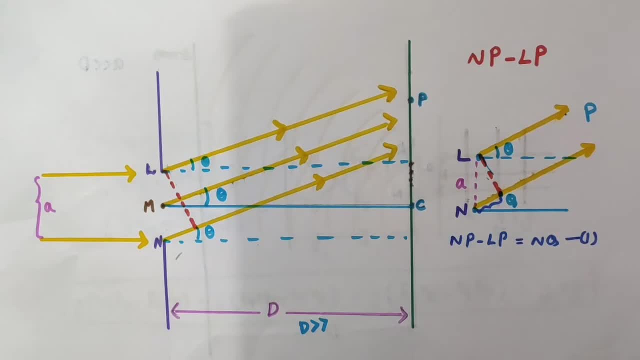 And I am taking this as equation number 1.. Okay, Now you see, this angle is theta. So what about this angle? This angle would be 90 minus theta, because this is a perpendicular line. Now, perpendicular line means from here to here the angle is 90.. 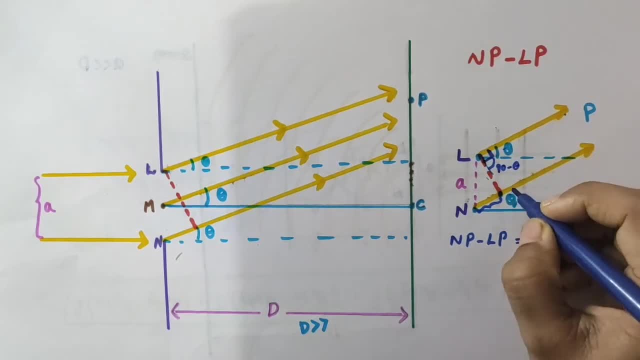 So if this angle is theta, this would be 90 minus theta. Okay, Now you see, this is the slit LN of width small, letter A. So I just drawn a dotted line here of length, small. So this is the slit LN of width, small, letter A. 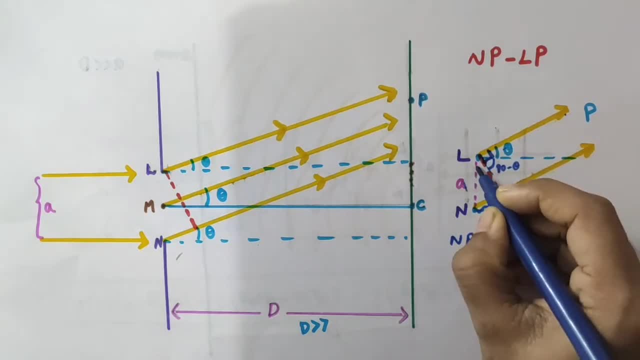 This is actually a perpendicular line with this one norm. So this angle, that is, this angle, would be 90.. If this angle is 90 minus theta, this angle would be what Theta? Then only theta plus 90 minus theta, minus theta plus theta cancel, and thus we will have the angle between these two. 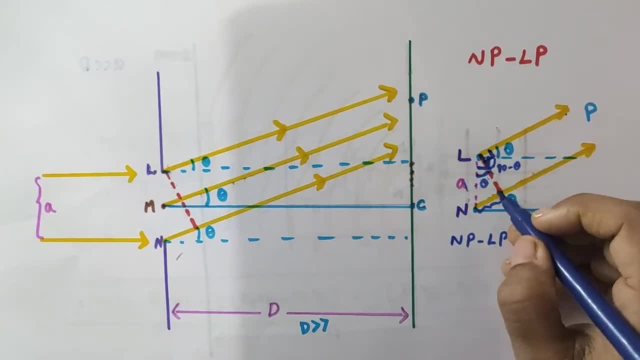 This green, I mean blue colored one and the pink colored one would be 90.. Okay, So here We have a right angled triangle, That is, This angle would be 90.. So here we have a right angled triangle. LNQ. 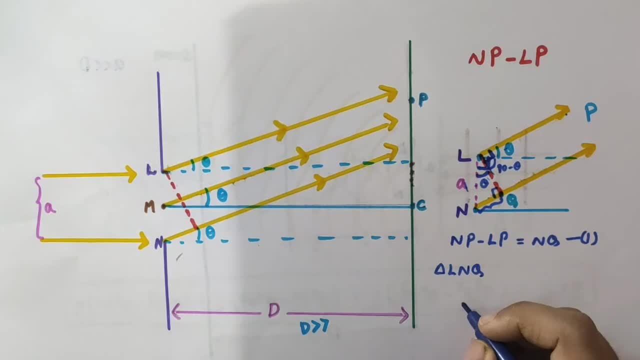 Alright, So I am considering that right angled triangle, LNQ. Alright, Then here, if I am calculating sine theta, what would be? that Sine theta is equal to opposite side. Opposite side is NQ divided by hypotenuse. 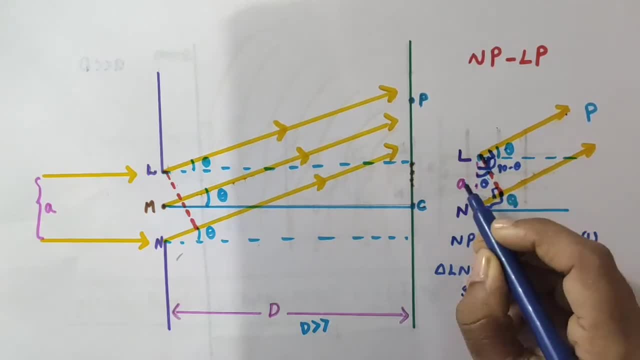 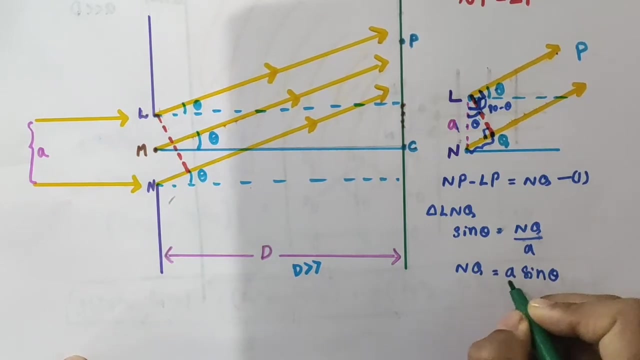 Hypotenuse is the side of the triangle which is opposite to the 90 degree. That is A Okay, So A Alright. So from this we can write: NQ is equal to what? A sine theta Alright. Now if we substitute this value here in this equation number 1, we will get the path difference as NP minus LP is equal to what. 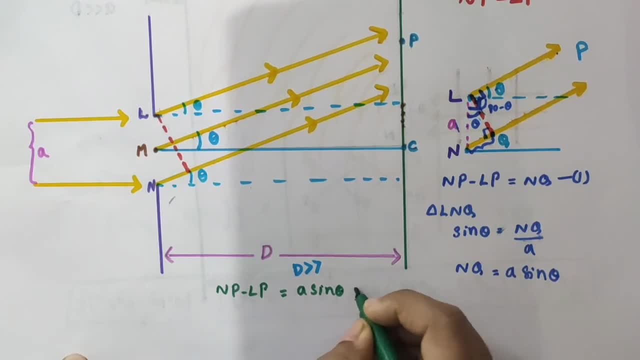 NQ is A sine theta. Okay, I am taking this as equation number 2.. Alright, Now for small values of theta, that is, if theta is very less sine theta can be approximated to theta. Okay, So this equation number 2 becomes: 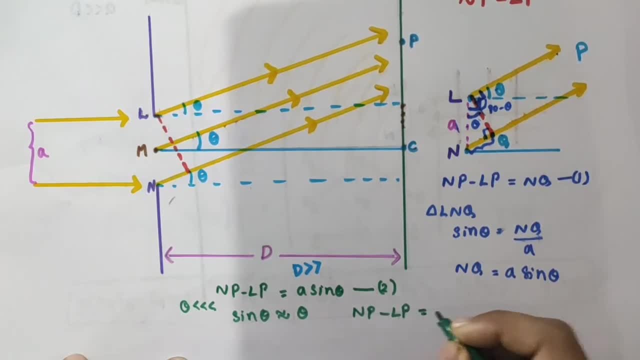 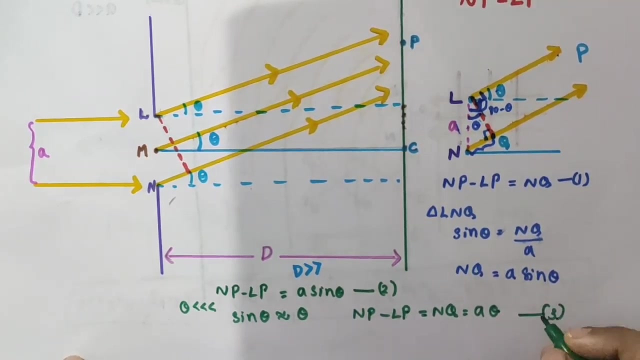 NP minus LP, which is actually equal to NQ, And that NQ is actually equal to A sine theta. But if theta is very less, then sine theta can be approximated to theta, So that is A theta. Okay, I am taking this as equation number 3..